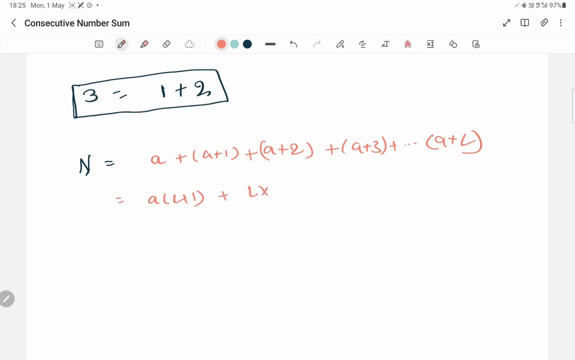 plus. this can be written as what l into l plus 1 by 2. we know the formula of summation of n consecutive numbers starting from 1. then uh can further subsist and reduce this to: we can take a left and n we can brought. 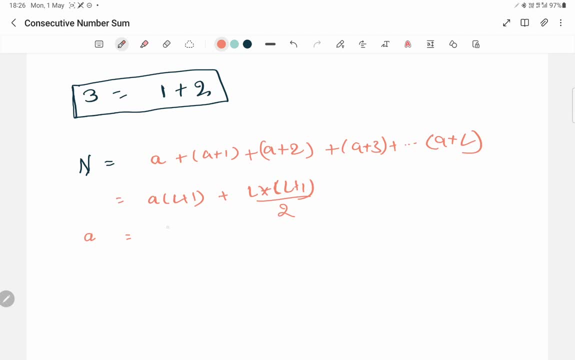 it right side, then it will become a equals to n minus L cross L plus 1 by 2. this will be the formula right. so when? this will be the formula it means when a is a natural number means sorry, yeah, when a is a natural number from 0 to any value. 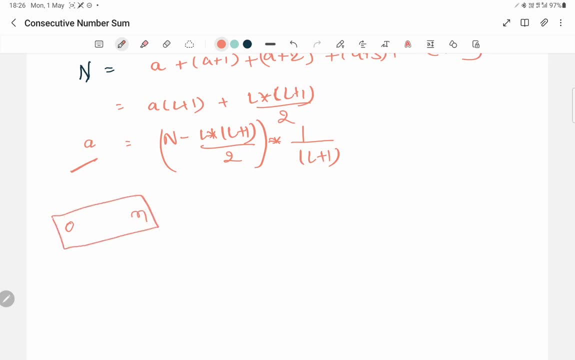 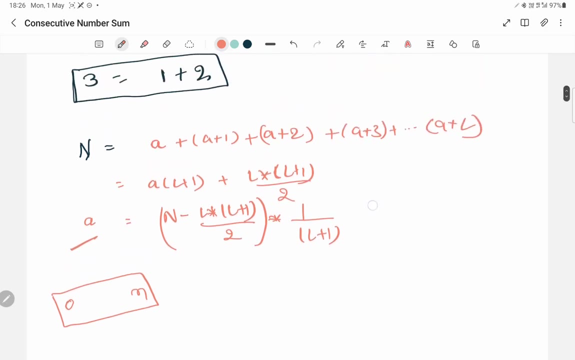 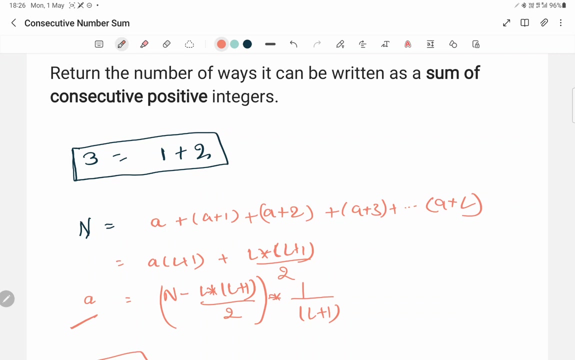 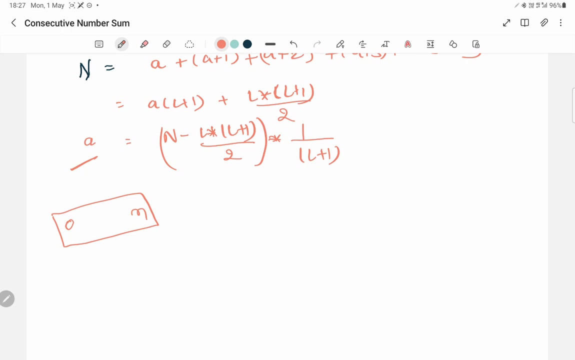 then we can say that, okay, this value is, whatever the value I am getting, that is, that will be a concluded as that the it is the sum of consecutive positive integers. n is the sum of consecutive positive integer, so so we can say that this value to meet, 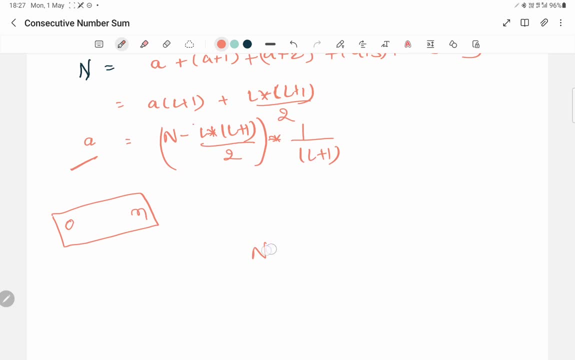 the condition n, sorry, not n L. into L plus 1 by 2 should be less than n, sorry, not n L. into L plus 1 by 2 should be less than n, sorry, not n L. into L plus 1 by 2 should be less than n L into l right and whole. 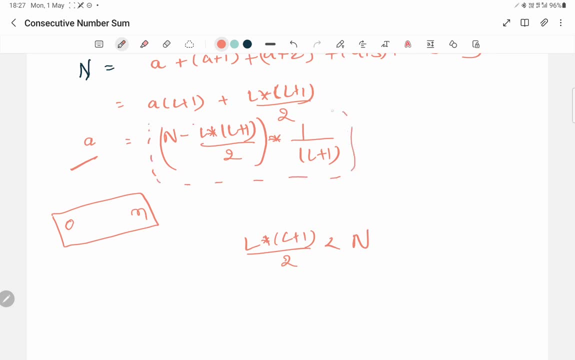 whole formula hold. this equation should give the output of output as a net, as an integer, desert value a, so less go the code. I think this is basically directly onto a formula, so you can directly apply the formula. that the only thing is how you are going to apply. that is important. so what actually we will do? 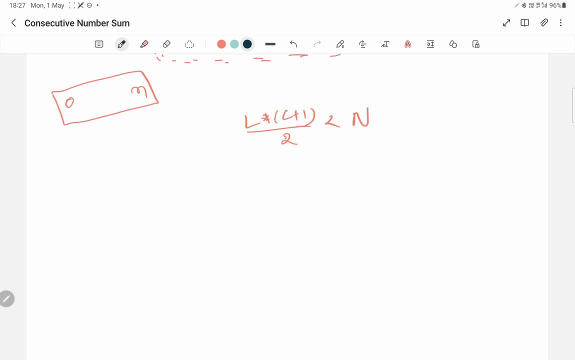 do is, initially, when L value is 1, then what will be the value of this? this will also be 1, right? so we can say that let assume it as a val, only right. and we will take one variable, I one, and let's say count also, count equals to one. 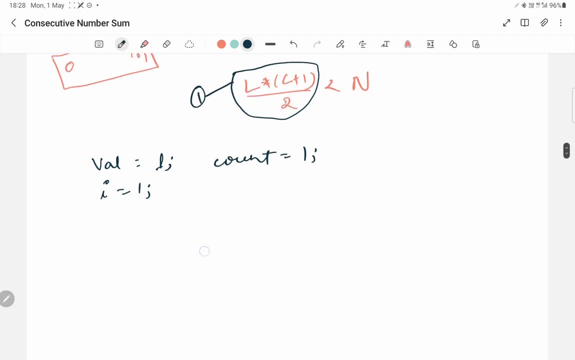 because when we have already added, so right. so although we can say and number, let's say n- is given. so we can say that when val is less than n, then the this looks like this. so we can say that when val is less than n, then this looks like: 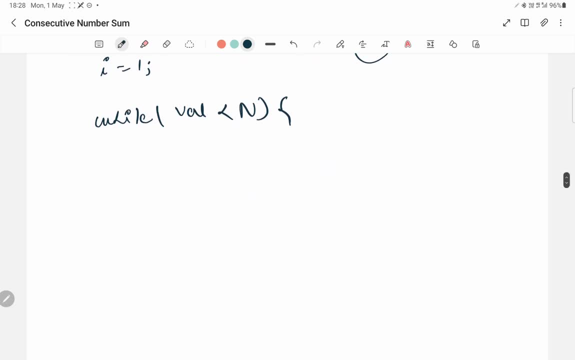 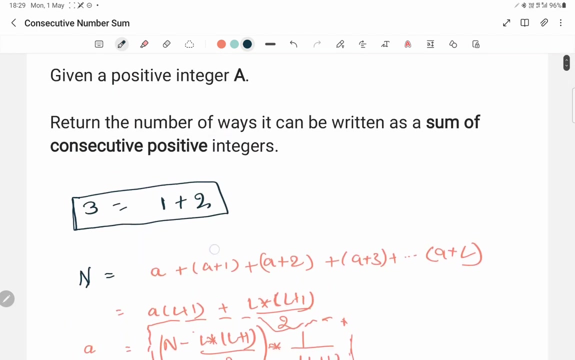 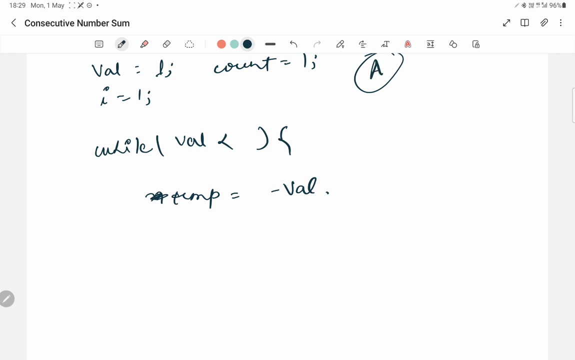 should run, then n equals to what I mean, some temporary variable, let's not, and it will confuse. so let's say temp equals to. I am saying a minus in equation now, I mean in quotient is given a right, so not n. so we will take a minus file and we can say that if temp minus, sorry, temp mod L plus 1, I mean. 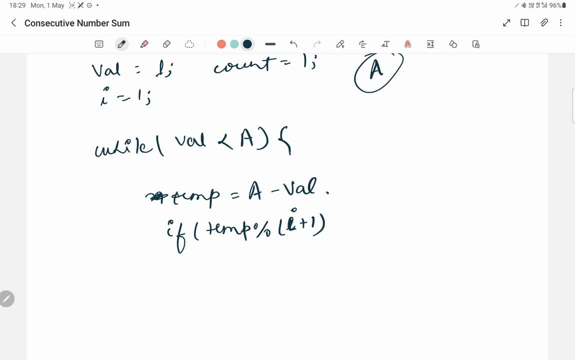 here it will be: I, I plus 1 is equals to equals to 0. then what count? plus plus, right, then I plus plus. we will increase that value of I and then we will have to change the value of val also. then val will become what I into: I plus 1 by 2, right. 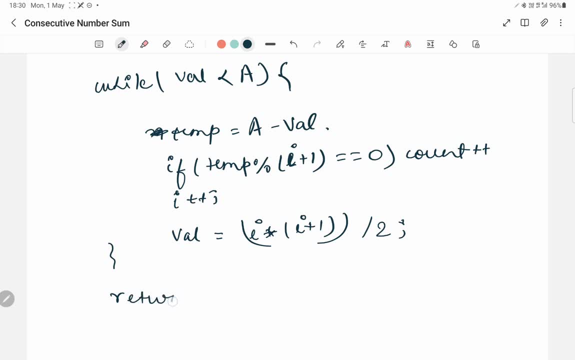 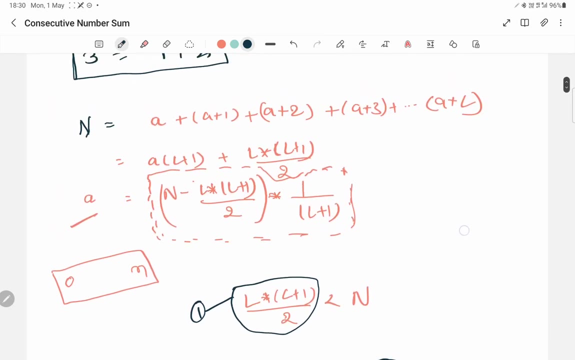 and finally, we will return the count and hope you have got this problem and solution as well. yeah, so thanks for watching this video. thank you very much.